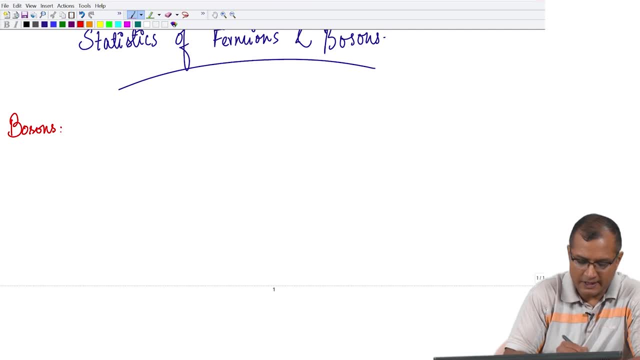 of bosons, And here we have already seen that these are classified as particles. So these are a defence unit of the bosons whose wave function, the wave function of the n particle system or the wave function of the n boson system- has an even parity. So this essentially: 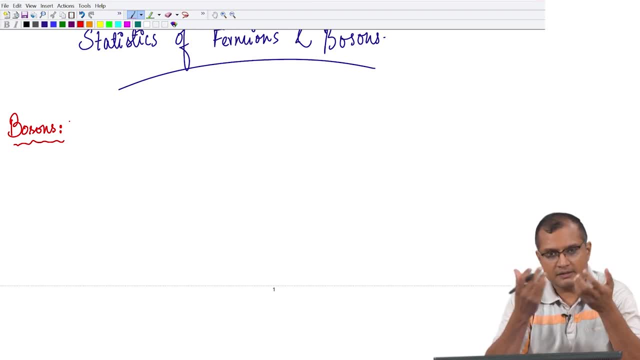 means that if I permute the particles in the system, the overall wave function does not change its sign, And this has natural consequences on the statistics it follows. 1. Dahae h. So the evenness of the parity operation allows an arbitrary number of bosons to sit in one. 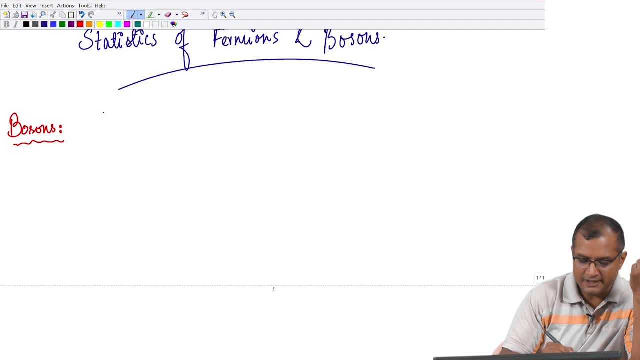 energy level And this is usually represented as the spin being in integer. so they are classified as integer spin particles and there is no restriction on the number of particles that can sit in a given energy level. I am going to say that as N j you know. 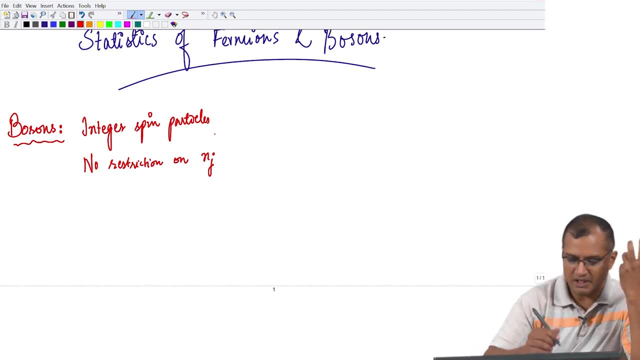 The number, density or the you know it can only be. it can be any number between 0 and infinity. ok. Number of particles in some energy level: j- ok, So I can write down the partition function for this system. Ok, Under constant NVT conditions. ok, for N bosons as summation over all the microstates that. 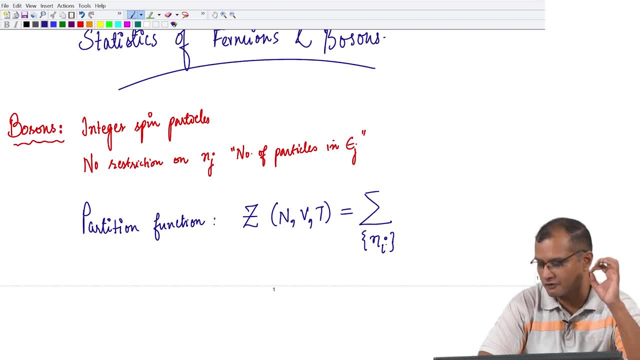 is the possible. you know values of these N? i's which constitute a single microstate and you sum over all possible values of these N? i's. Ok, So you can write down the possible values of such N? i's into e raise to minus beta. 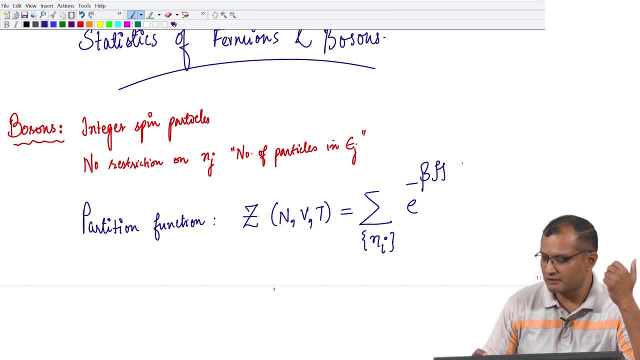 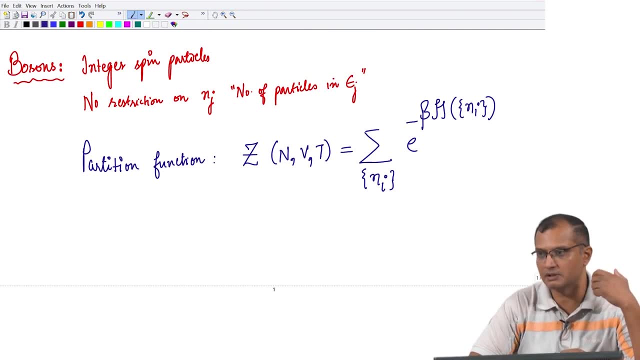 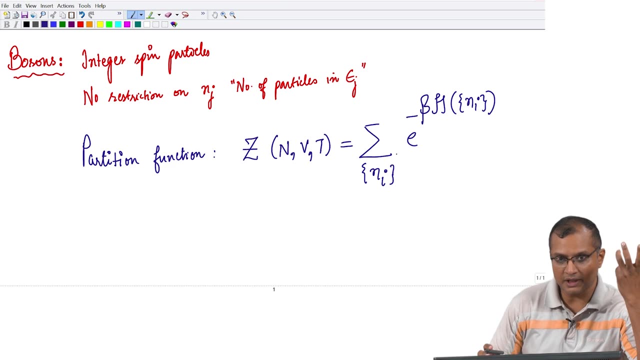 the Hamiltonian. So this is your, the Boltzmann factor. What is meant by summation over all possible excitations N? i? well, this summation is over all microstates. ok, So let us take off. you know, take one microstate here. 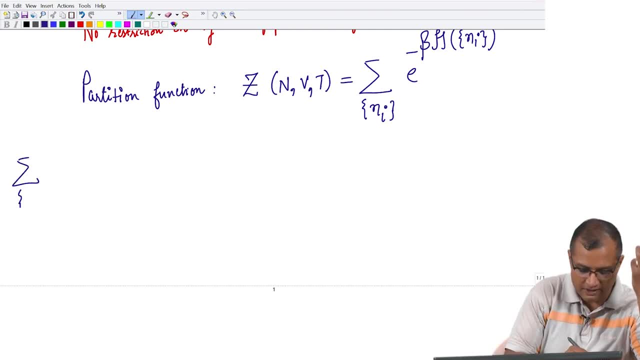 So the meaning of, So the meaning of summation over N? i is basically the fact that you know your sum over microstates. ok, So what is the sum? how is the sum implemented? how do we visualize in our heads this sum? 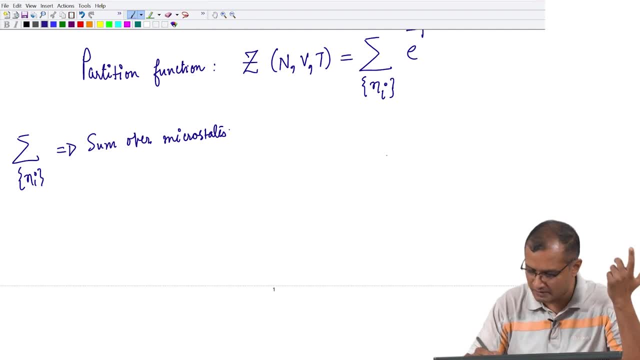 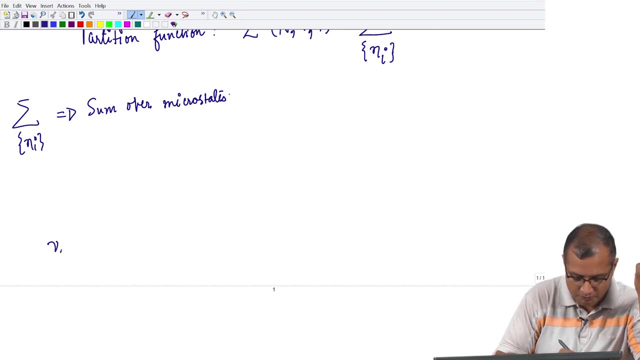 Well, you take one microstate, So I am going to write down one microstate. Let us say I am going to write down microstate Ok. So I am going to write down microstate mu 1.. In this microstate you could have the energy levels. 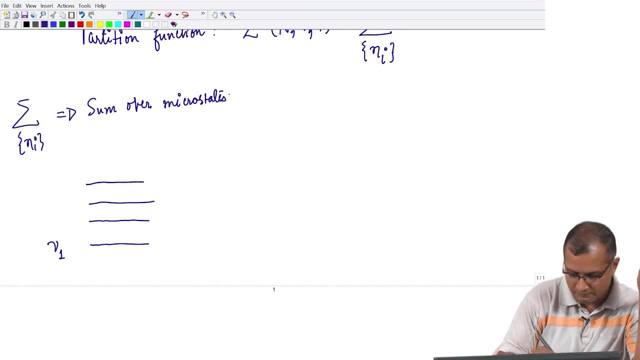 Let us say, you know, you can have energy level 1,, 2,, 3,, 4 and so on in infinite energy levels. Ok, So the number of energy levels are not you know, they are basically uncountably large. And let us say in the microstate mu 1, I am having three bosons sitting in the first level. 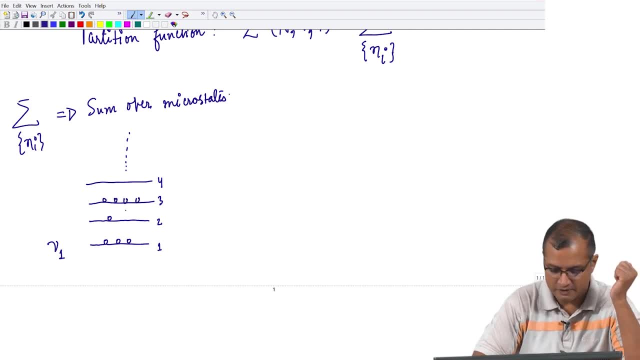 one boson sitting in second and you know four of them sitting here. So basically, for the microstate mu 1, I have N 1 equals to 3, N 2 equals to 1, N 3 equals to 4, and so on. 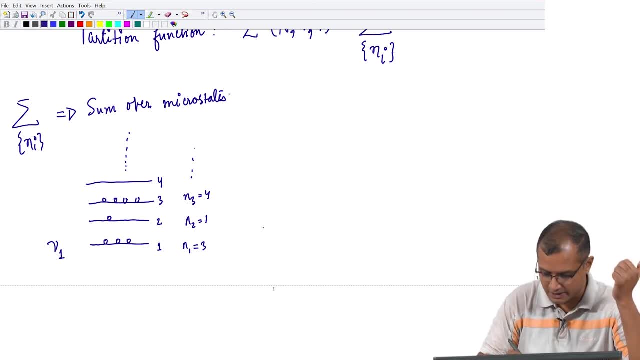 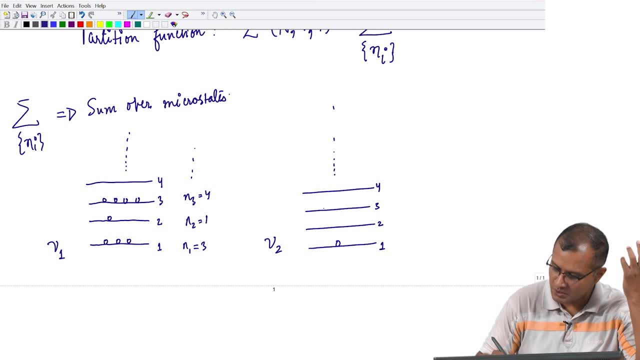 say, one particle sitting here, nothing sitting in 2, you got 5 sitting here and maybe 2 sitting here. So now my N 1 is 1, N 2 is 2.. N 2 is 0, N 3 is 5 and N 4 is equal to 2, and so on. 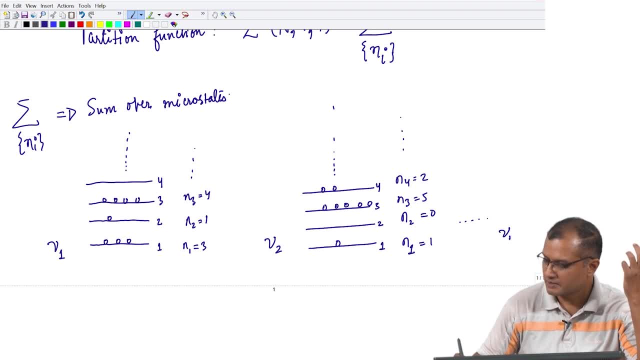 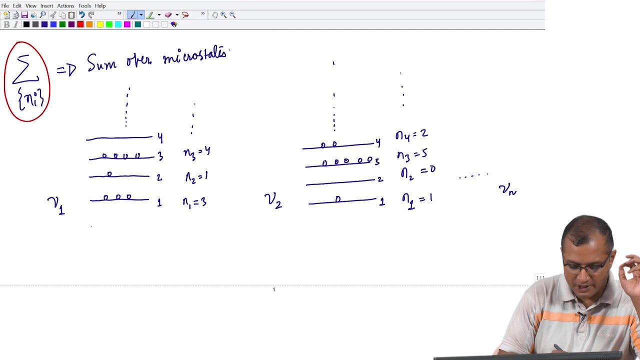 So this way you can change your microstates. So the summation over microstates that I am I have written here is basically the summation over all possible sets of Ni. So, for example, this would be mu 1 microstate would be the set you know. 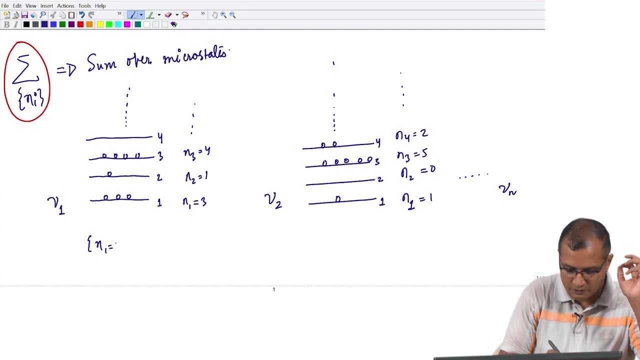 Ok, You know, with the values N 1 equal to 3, N 2 equal to 1, N 3 equal to 4, and so on, Then my set of excitations become N 1 equal to 1, N 2 equal to 0, N 3 equals to 5, N 4. 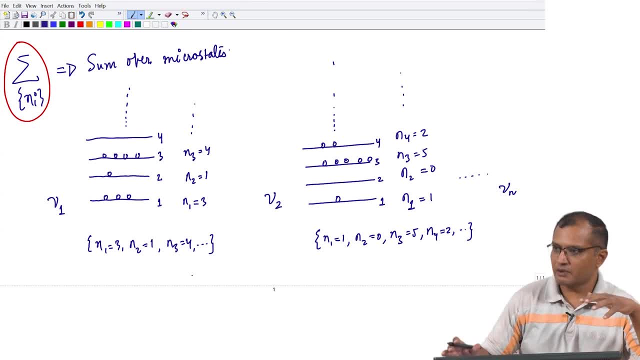 equals to 2 and so on. and with the third microstate my set changes. So that is the meaning of summation over all sets of Ni. You take one set of Ni's that is constituting your one microstate, Then the set change. 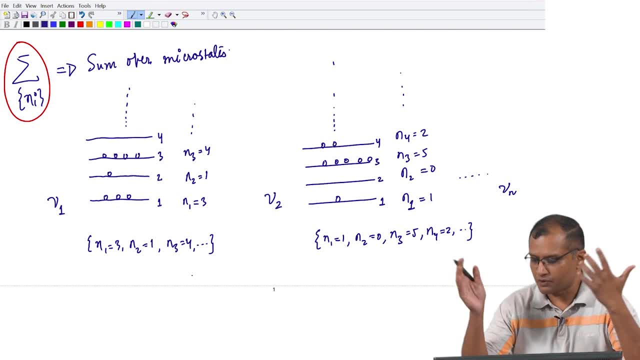 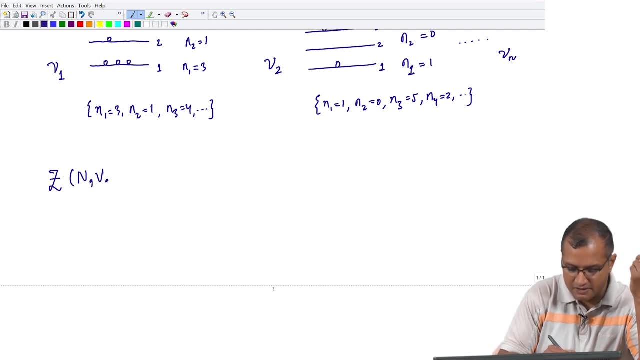 So you are now looking at a different microstate and so on and so forth. So that is the meaning of our partition function at constant NVT conditions. So you have summation over all the set sets of Ni's. and our Boltzmann factor was e raise. 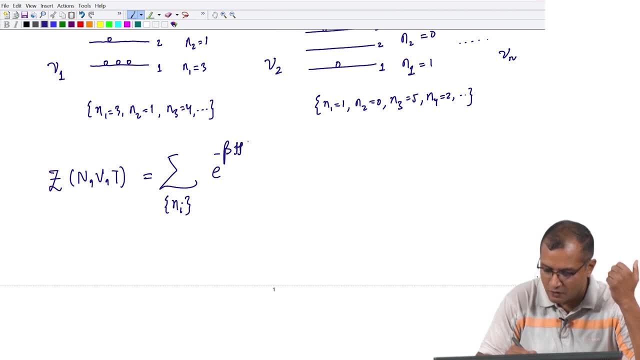 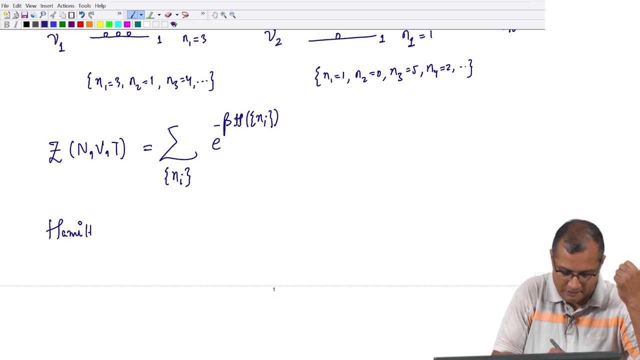 to minus beta. the Hamiltonian of that particularly chosen set, Ok, In the summation. ok, Now the Hamiltonian of the microstate ok, is given by nothing but well, the energy of the state multiplied by the number. Ok, Ok, Ok. 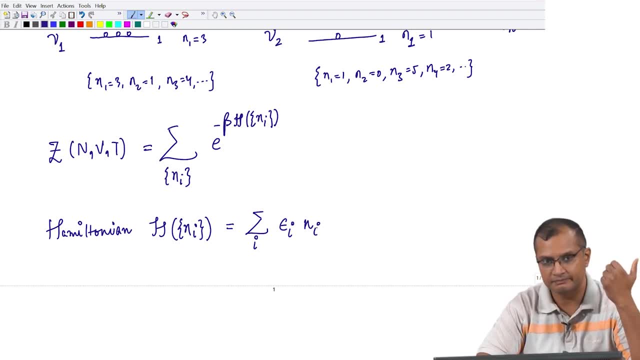 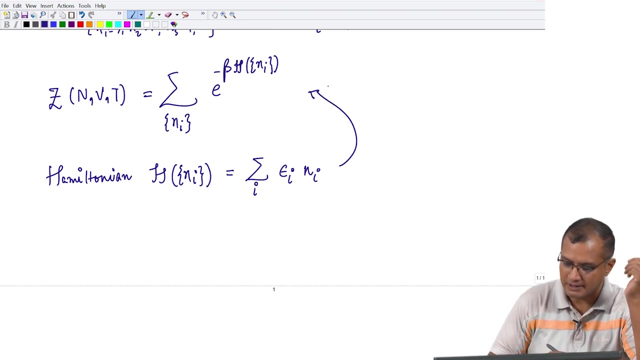 Ok, So the number of guys sitting in that state? ok, I will run from 1 to infinity, because you have infinite energy levels in the system. alright, So let us plug this value here And now. I can write down my canonical partition function as summation over all possible sets. 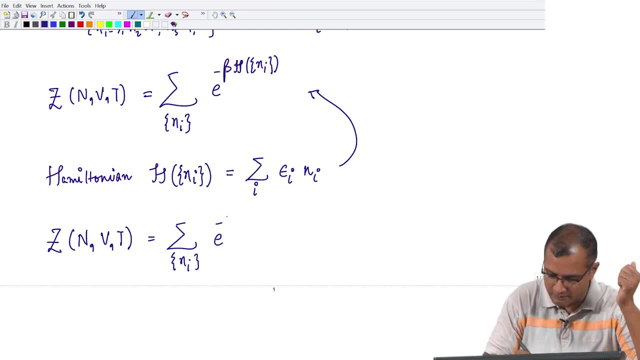 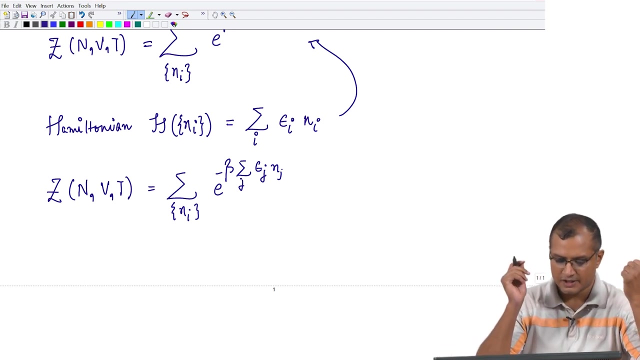 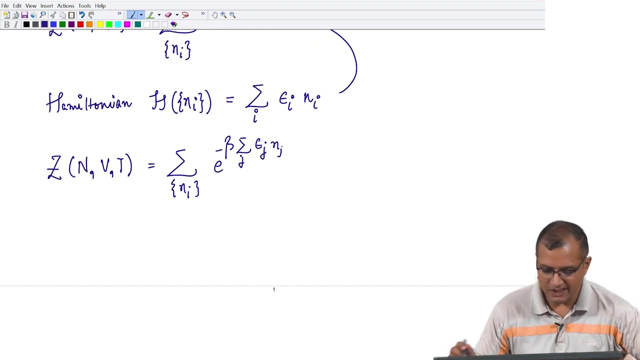 of Ni's. Ok, So I have taken the values. Ok, Ok, So I can write it down. So j is min. then for that microstate you compute the Boltzmann factor. Now this can be written as: 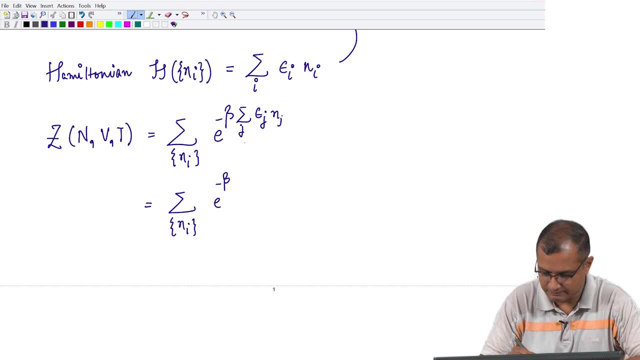 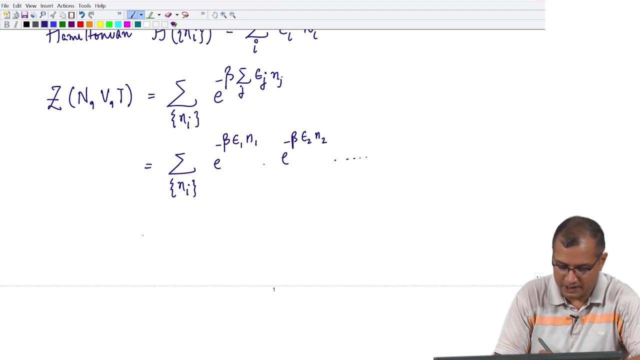 e to the power minus beta. ok, There are infinite terms here. but there is now a problem which becomes clear, So I can write down this as you know, the product of these exponents- These are taken here outside, and the sum for each value of j that I take, suppose j is 1- 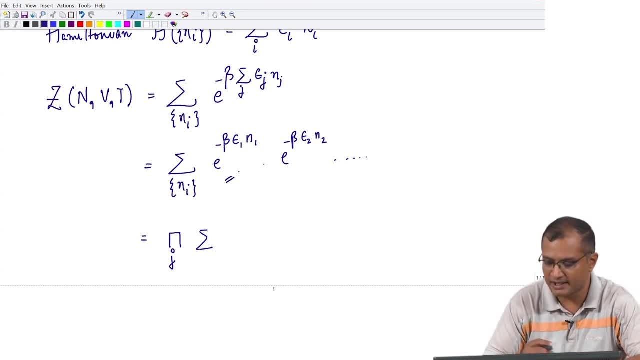 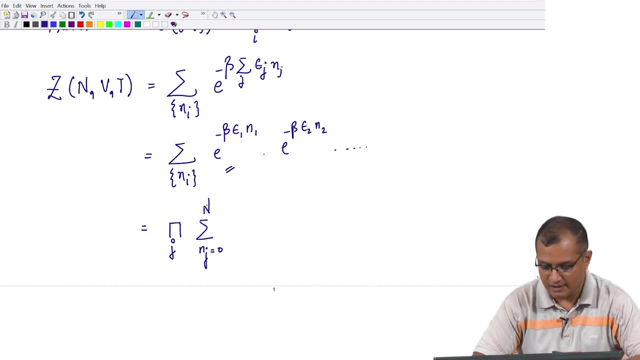 then I have this particular thing, but it has to have a sum over all the ni's. ok, So then I will take my nj going from 0 to n, because I have n fermions in the system, and this is basically e to the power minus beta. 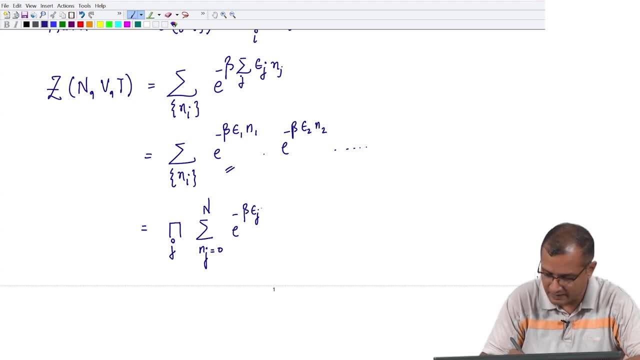 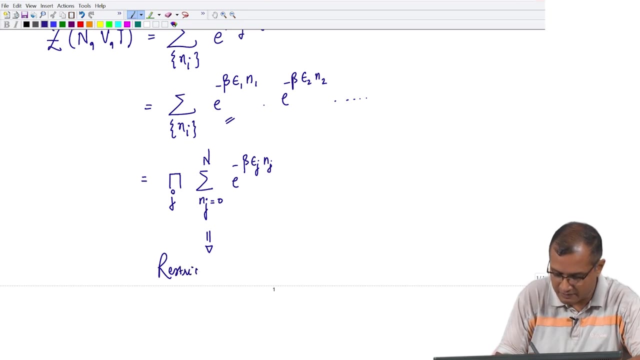 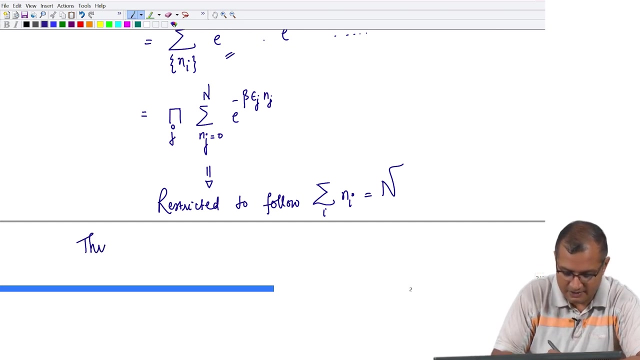 So e to the power minus beta, e, j, n, j. and it is very difficult to perform this sum simply because I have a restriction here. The sum is basically restricted to follow a constraint. the total number of particles is very hard to perform, meaning being the label n, j, which is the occupancy of jth level. 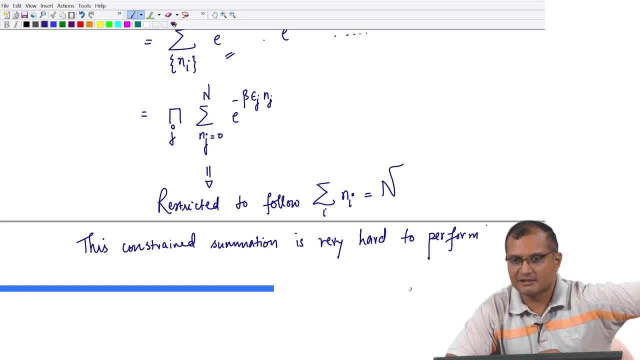 cannot be independent, taken from 0 to n, for these exponents. Suppose I take n j as n by 2 for the first exponential, the next exponential cannot have n j, anything other than you know. what I am left with is basically: I cannot take it as n by 2 plus 1 and I have got infinite. 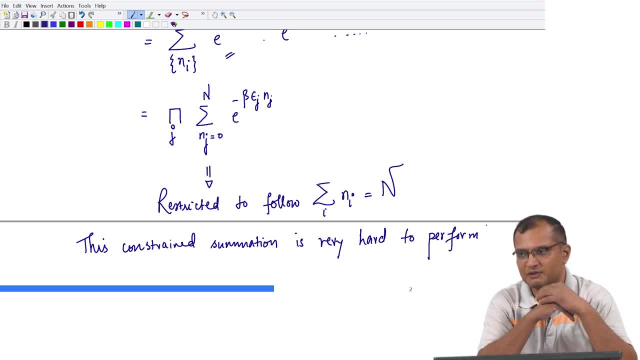 number of exponentials there. ok, So for each one of them the label n, j cannot take independent values. They are constrained to sum up to n, which is the number of particles in the system. So I cannot perform this summation. 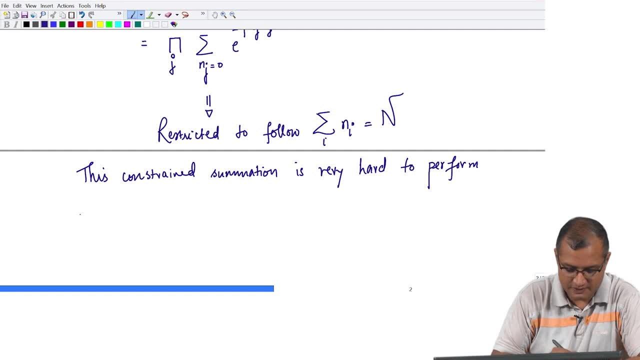 It is very hard. So what is the solution? So the solution is to shift the problem to the grand canonical ensemble, where n can change, ok, but it will keep the chemical potential constant. So I am going to go to the grand canonical ensemble, where number of particles 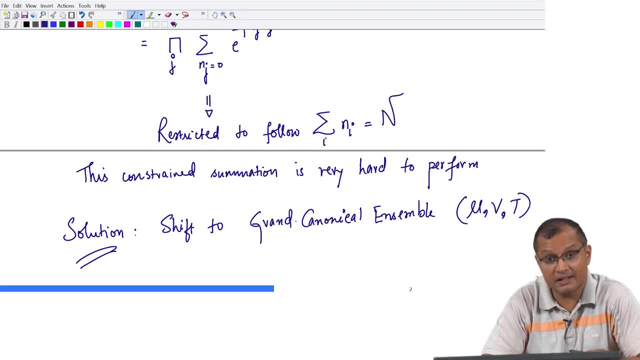 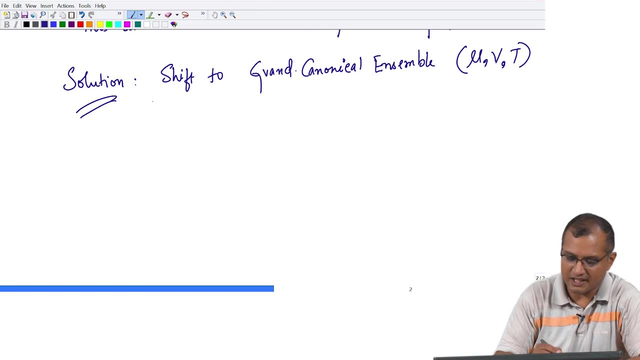 in the system can change. This sum becomes unrestricted now. but now I have to conserve the chemical potential. So let us shift to the grand canonical ensemble, which means now I will be computing the grand canonical partition function, indicated here by two horizontal crosses on the function. 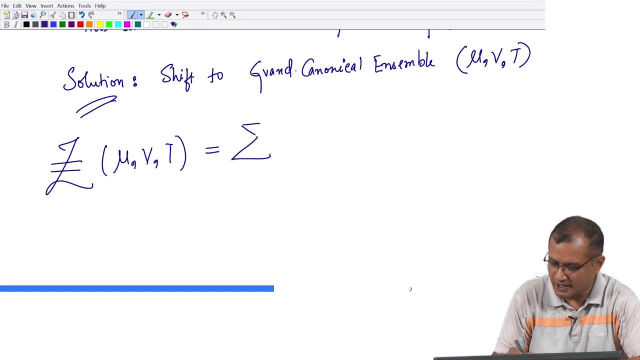 z and as usual here I am going to write down my partition function as summation over all the microstates into e raise to minus beta. a Hamiltonian of the microstate that is chosen by the summation here. ok, Now the Hamiltonian of the microstate in the grand canonical ensemble. 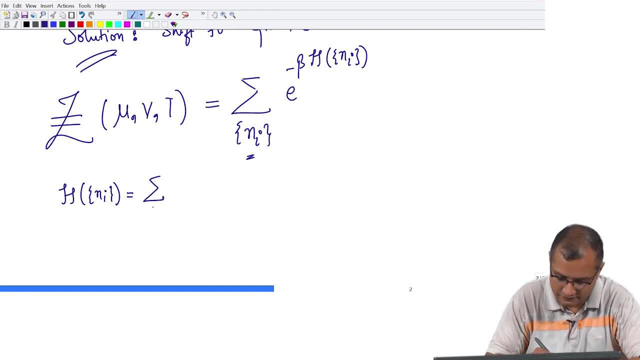 is nothing but summation over all the values of energy levels times the excitation of the level or number of particles sitting in that level and multiplied by energy of that level minus n j times chemical potential, because we have taken summation n j as n? n for that. 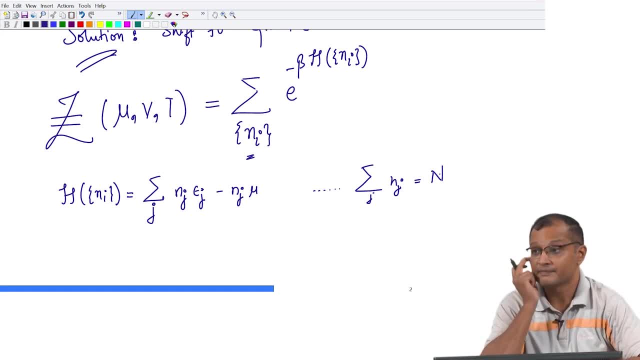 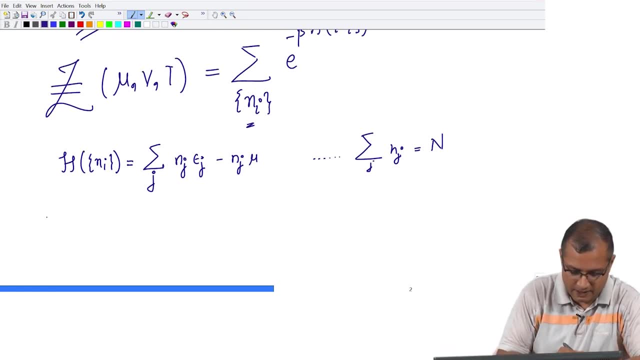 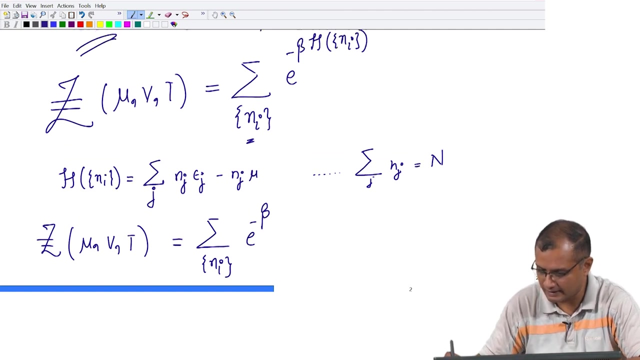 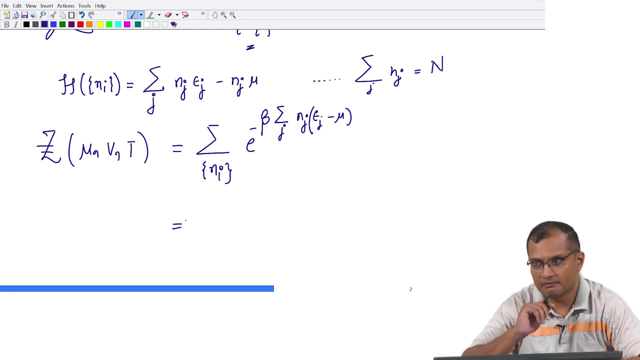 particular of microstate, because n itself is now changing. ok, this in the above expression, our grand canonical partition function now becomes summation over all the microstates. e raise to minus beta, and I am plugging the Hamiltonian here: summation j n j into e j minus mu. as usual, the exponent is a sum, So that becomes product outside. 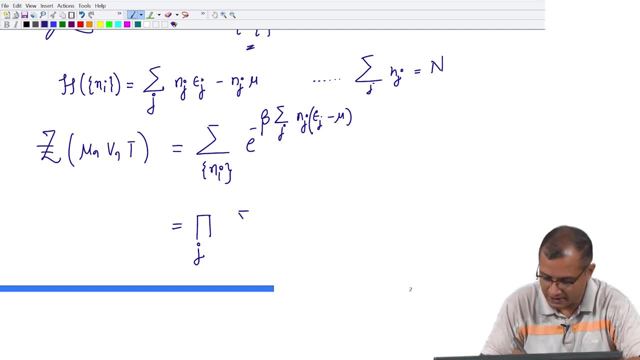 so then I have: for each j, I will now take an unrestricted sum. So this is the meaning of the unrestricted sum. So unrestricted sum here. now, for each exponential, my n, j can go from 0 to infinity, and this will be e to the power minus beta. So now you have no problem. So this is now an unrestricted. 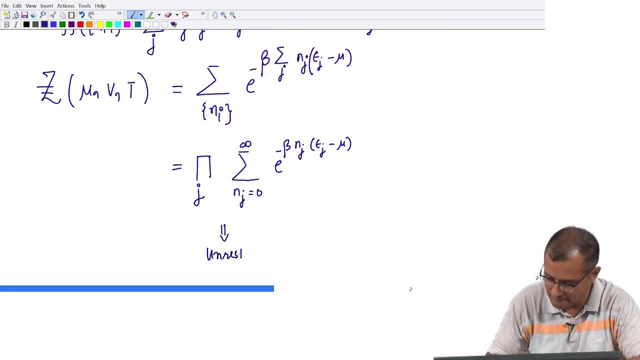 sum. So I can take in each exponent my label going form 0 to infinity, which I could not do previously. So if you take 0 to infinity then you can do anything in the second one, because your n has been. you know you have to conserve the 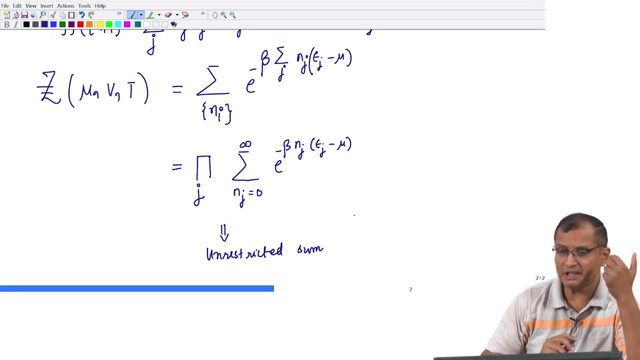 total number of particles. But here I do not have to conserve a number of particles. my n could be actually infinity. it could go up to infinity, which means each n j which is independent of the other exponent can run from 0 to infinity without getting affected. 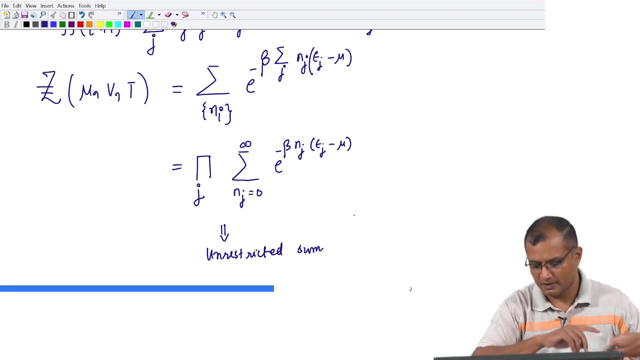 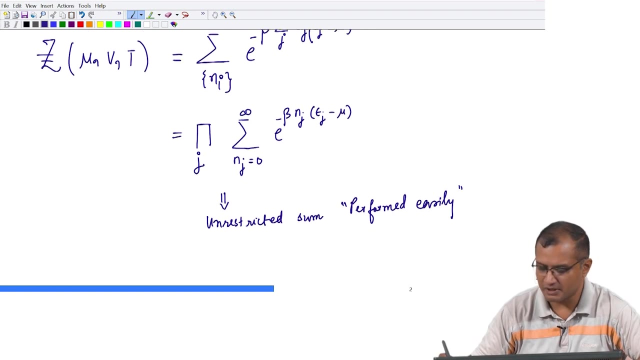 by the label in the next exponent. So this is now I understood, some which can be performed very easily because I am not conserving number of particles anymore. ok, In the grand canonical ensemble, number of particles is not conserved. what is conserved? basically chemical potential. 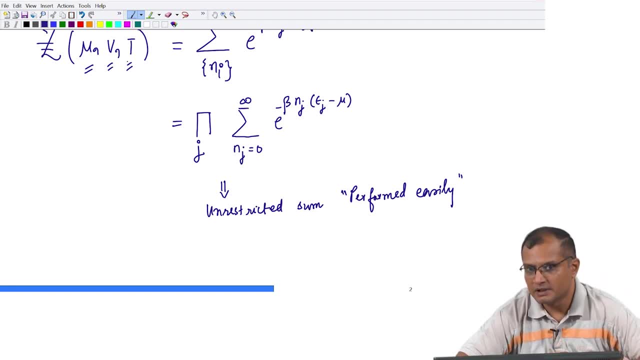 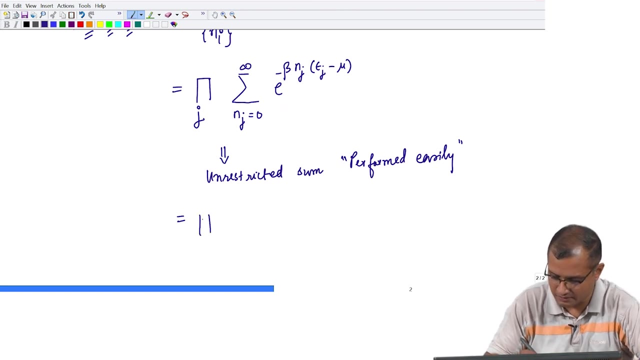 volume and temperature, and that allows us to compute this sum in an unconstrained manner, which we could not do previously. ok, So then I can write down this as: So let us just pi j, sum over all the j's, and for each j that I set outside, I am going: 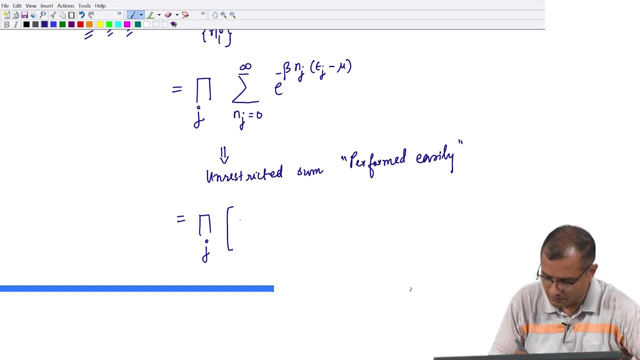 to write this sum inside for a few terms. So I am going to take the first term, for j equal to 0, n, j equal to 0 is 1, then the second term is minus beta, E, j minus mu and n, j becomes 1.. 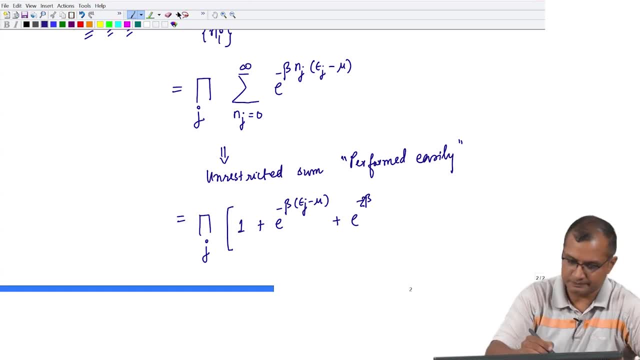 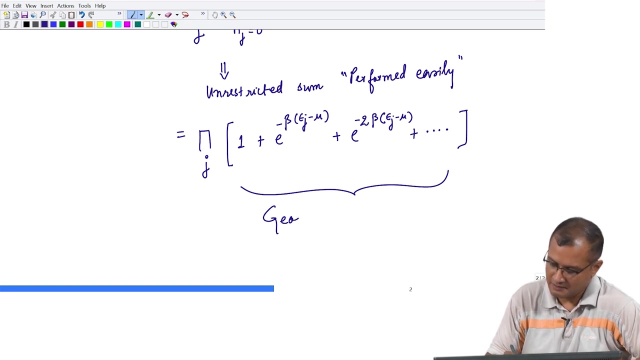 And for the third term. So it is E raise to minus twice beta, and so on. you have infinite terms here. ok, As you can see, this is a geometric series with the common ratio r As e to the power minus beta, E, j minus mu, ok. And the ratio of the successive terms. 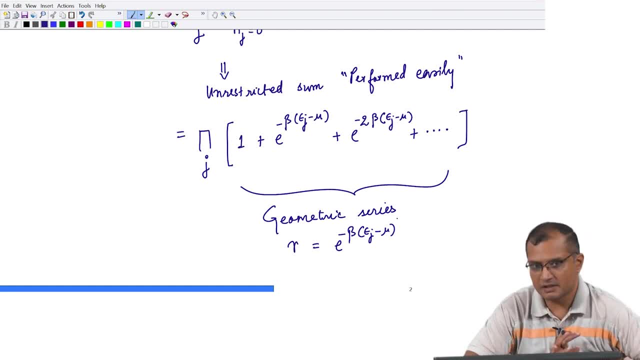 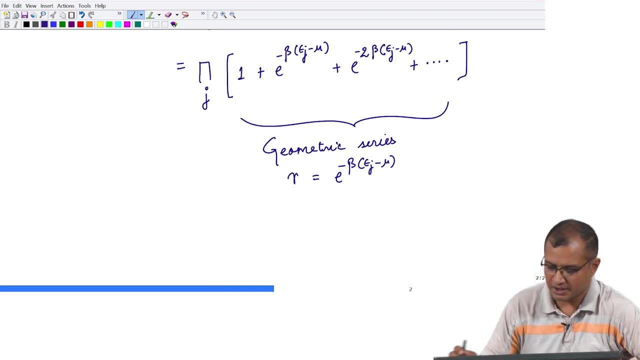 in the limit n going to infinity, converges for any value of beta, E, j, n, mu. So this sum converges to the closed form 1 upon 1 minus the common ratio, which is 0, n, j equal to 0. So this is a geometric series. So this is a geometric series. So this is a geometric 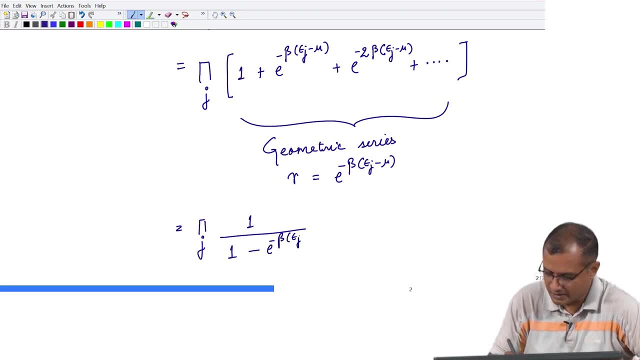 ratio which is E raised to minus phi, 0 plus beta E j n minus mu, is equal to 0, n to the power minus beta E j Kurt. as e raise to minus E j n minus mu e to the power minus beta E j y minus mu, that is the converged sum, fine. 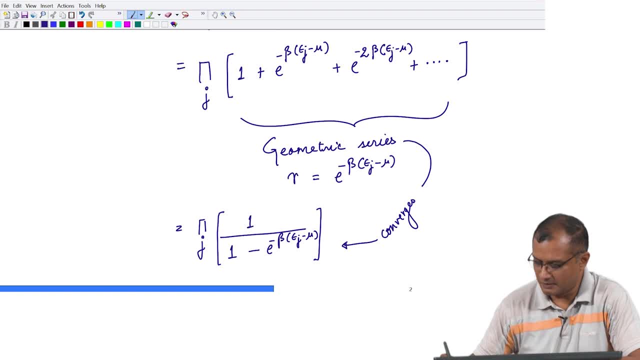 So that is more like only one statement. Now, is there any other question? Q torch, Something else? Okay. Intersection mention: Okay, So trade section. Okay, So trade section. Good bye, bye, bye, good bye, bye, and I have 2 more questions now. Yes or No? You have the易. 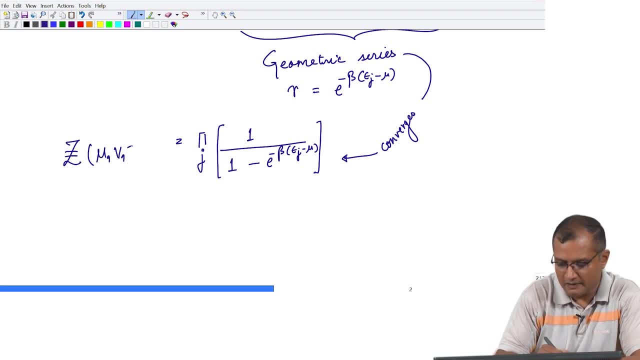 grand canonical partition function and thank the for the fact that, you know, the number of particles was not conserved and I could perform this sum in the partition function in the unconstrained manner. So before we proceed further, we would like to state here that the grand canonical ensemble is hence the natural choice of ensemble when 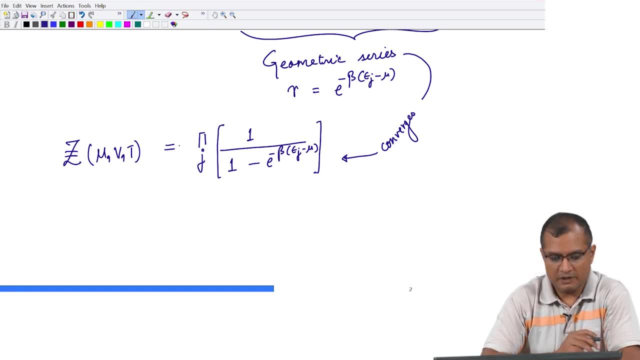 you are doing quantum statistical calculations. So when people say it is the ensemble to do correct enumeration of states, well, they are also saying this because it is also more convenient to compute the partition function. So the fact that I could enumerate the states properly, which is due to the fact that the sum was performed in an unconstrained manner, 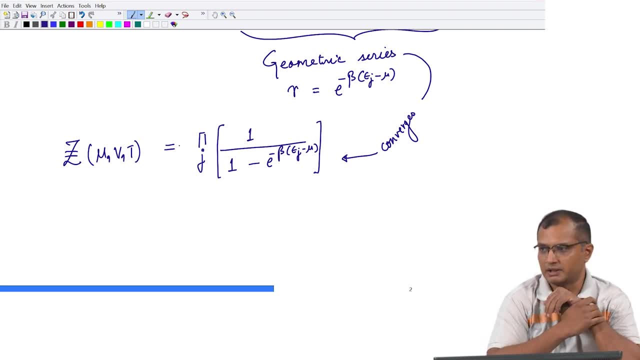 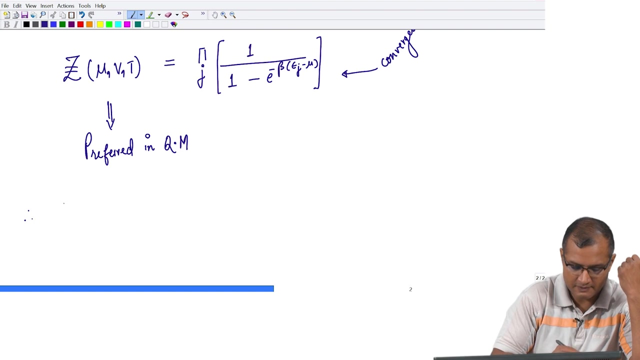 makes the grand canonical. So this is the grand canonical ensemble, a preferred choice for doing the calculations, ok. So that is why this is the preferred ensemble when you are doing a quantum statistical mechanics, ok. So then let us take a logarithm on both sides which we will be using it in. 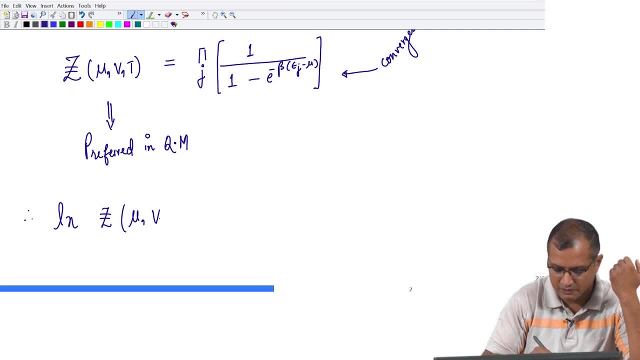 the corresponding order. So this is the difference between classical to, between quantum and classical statistical mechanics. So let us just make a small note of the result. if you take logarithm on both sides, what we get is nothing but minus. the logarithm of the products become sum. So 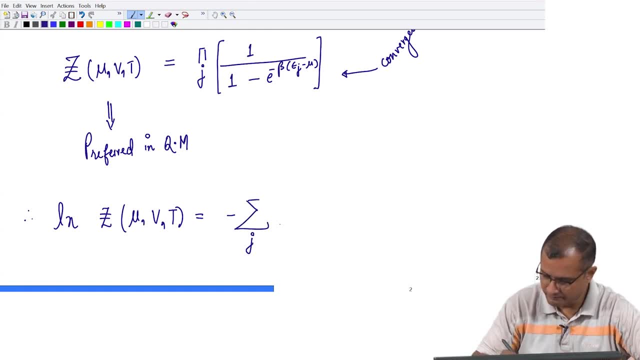 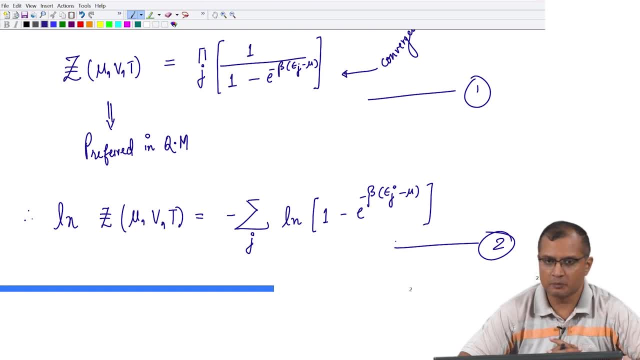 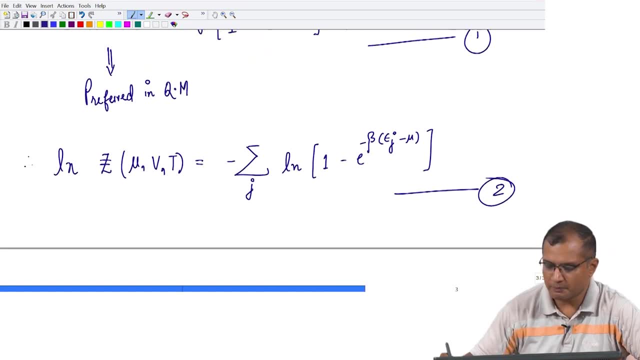 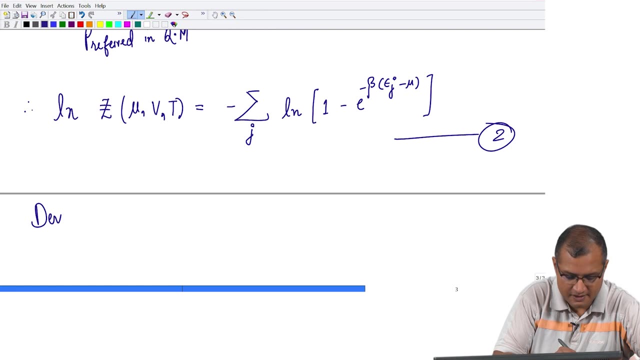 a position to compute or to form these statistics of bosons. So this discussion was for bosons, So I am going to derive the average occupation number of bosons in some energy level j. So deriving the statistics is now very straight forward. it is very easy now and since you 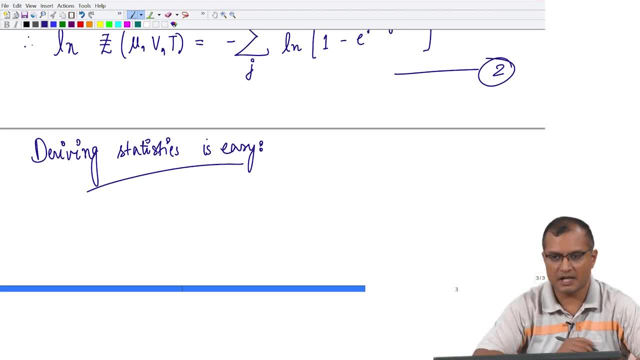 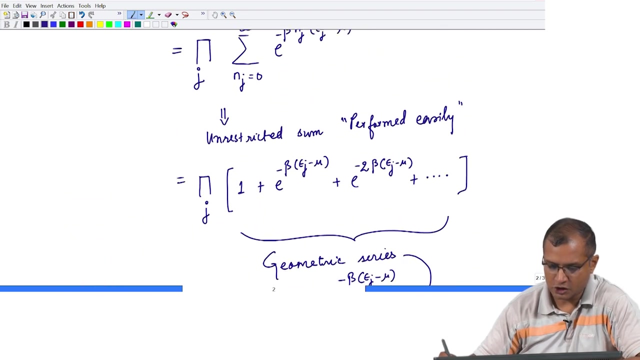 have followed the lectures in the first 2 chapters. you know how to compute average of any quantity if you know the distribution function in that corresponding ensemble. So I know that my partition function is represented here. either you can take expression 1 or 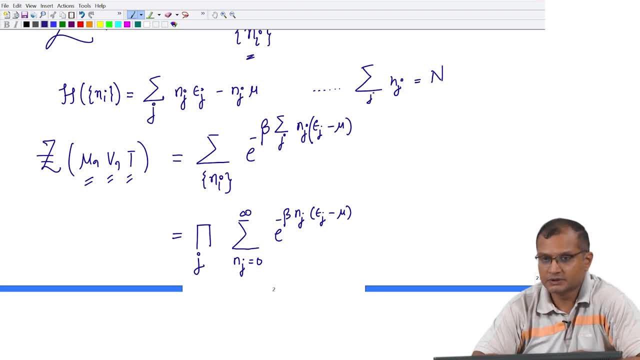 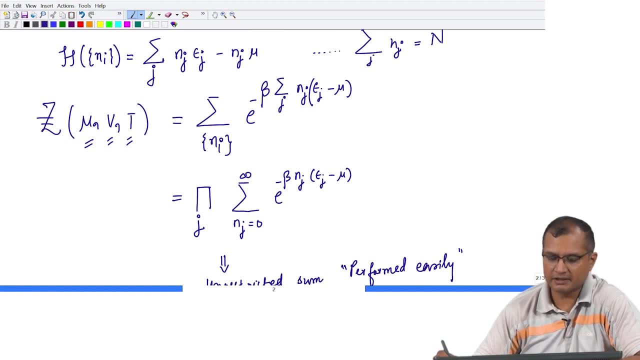 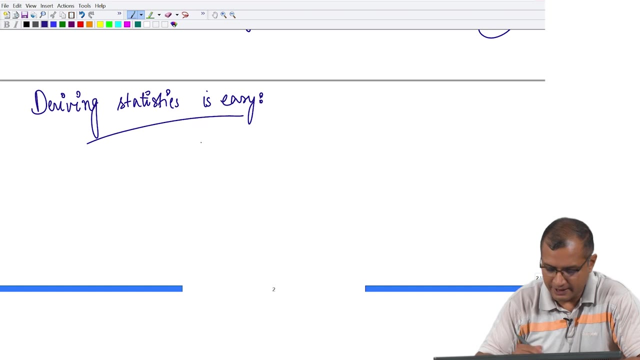 you can take the first expression here. So I am going to write down the. if I know the partition function, then certainly I know the probability of finding the microstate n? i? Ok, So certainly I know the probability of a microstate, some collection of these n? i's. 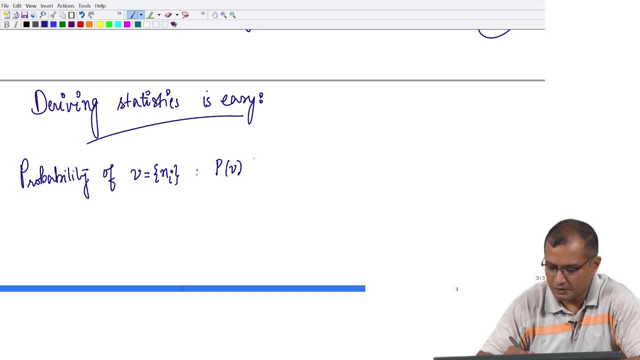 is basically P of nu or P of these n- i's ok- which constitutes a single microstate and the probability of this. So the probability of this single microstate is nothing but e raise to minus beta, the Hamiltonian of that microstate, ok, So therefore, if I want to know the average occupancy of 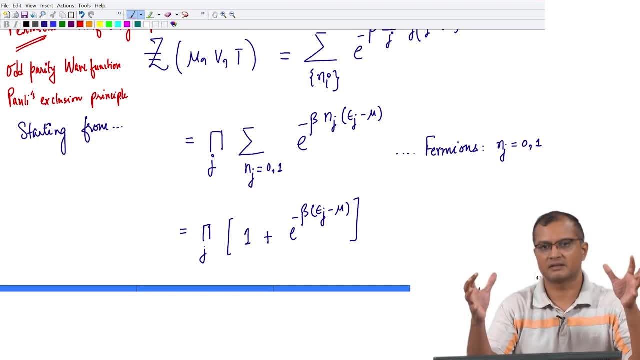 bosons and fermions differ from each other in the in the sense that one system has a wave function, that is, that has an even parity. the system of bosons and the system of fermions has an odd parity, which means the parity operator for fermionic wave function has an 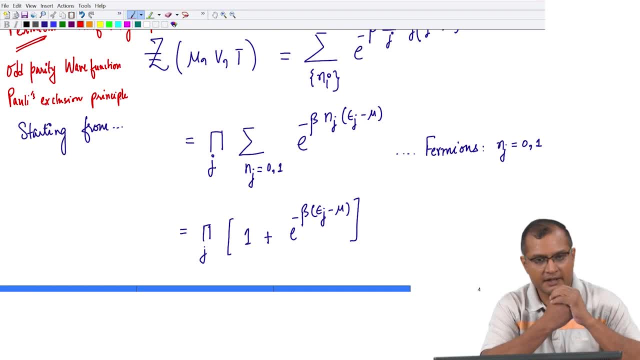 eigenvalue minus 1, whereas the parity operator for the bosonic wave function, you know, has a a bosonic systems has an eigenvalue minus 1.. So this basically means the following: that every time you permute 2 particles in a fermionic 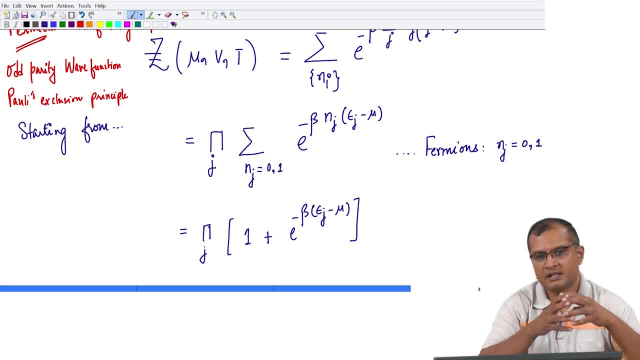 system, then the overall wave function incurs a negative sign. So that basically means that you cannot, like we saw in the last lecture, you cannot take 2 particles to be in the same level, because that would make your slater determinant to be 0.. 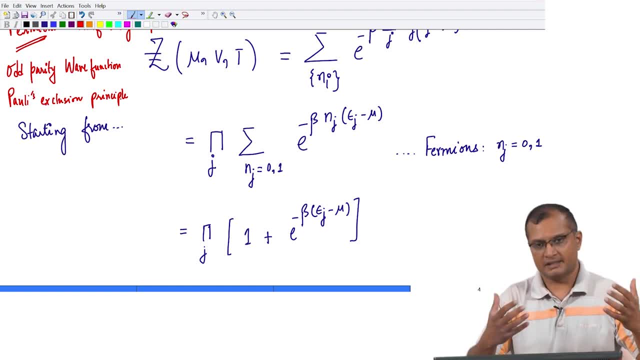 And that is the manifestation of Pauli's exclusion principle- that you cannot. your wave function will go to 0, which means you cannot see a realization where 2 particles are sitting in the same level. it will make your wave function to go to 0. So the system, 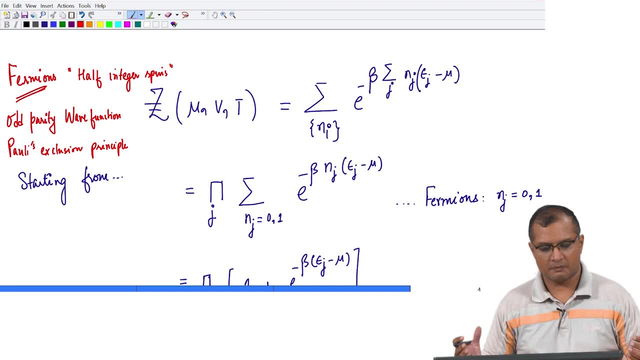 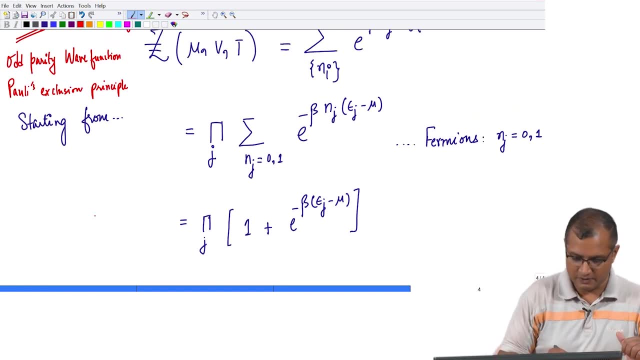 of fermions, half integer spins, because their odd parity wave function and they follow Pauli's exclusion principle. So this definition of the grand canonical ensemble. So we were doing the statistical mechanics purely from the directions from quantum mechanics and that has led to this. 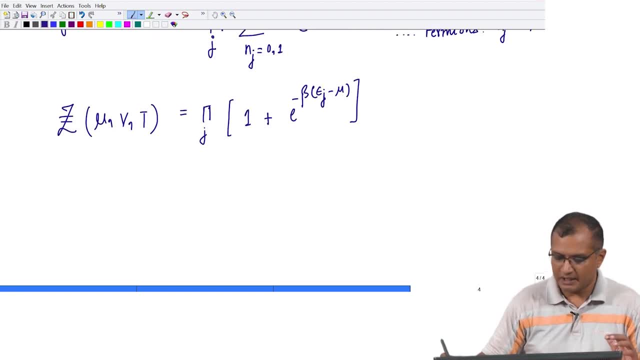 stage, and I can now take the logarithm of this, and this would be nothing but summation over j's ln 1 plus e raise to 1.. 這樣 I can do that, and so I can write. 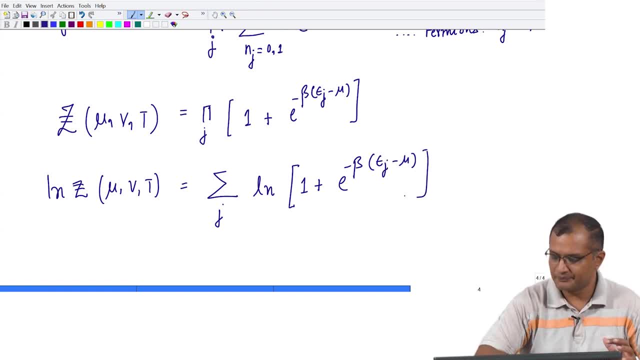 I can do So down here. let us say: meno n j bother острih. now this: the problem is that we will now't write the minimum reach of p m l to negative, less than or equal to minus beta e j, minus mu. ok. So therefore, as usual, if somebody 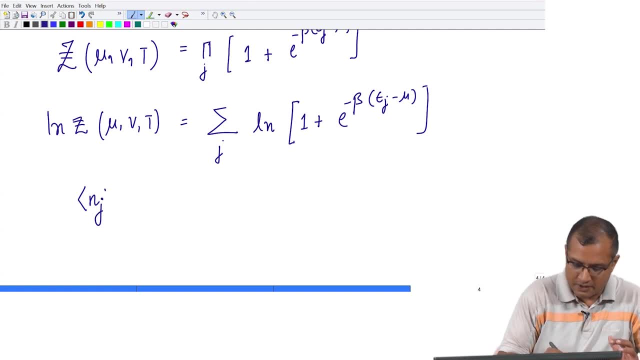 is interested in the average occupancy of fermions in some level j, then this is nothing but summation over all microstates. I need to sample n, j in this distribution like this. So I do not want. 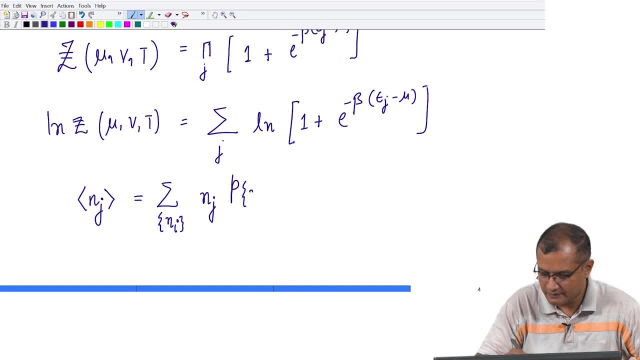 of microstates. ok, And as before, I know that this is nothing but e to the power minus beta. the probability of finding a system in a microstate is given as the Boltzmann factor divided by partition function. So this is my Hamiltonian divided my by a partition function. 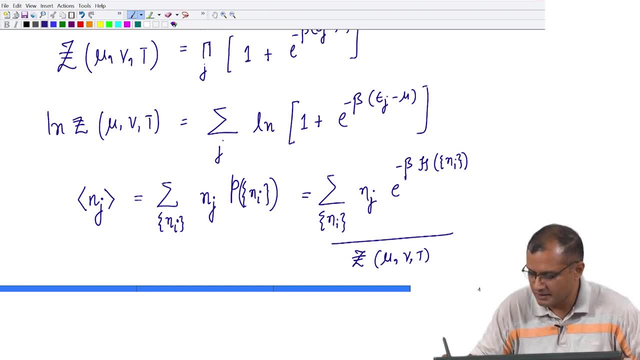 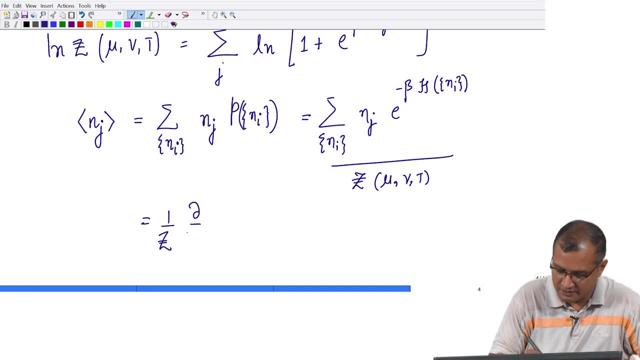 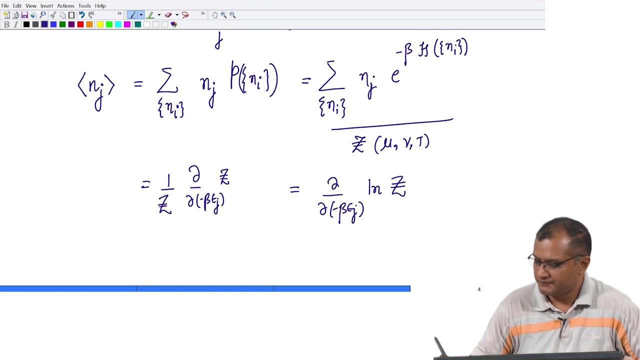 ok, And hence mathematically this is nothing but 1 upon partition function, d over minus beta e j, as before The partition function. So this is nothing but d over d minus beta e j of logarithm of the partition function. but now I will use the derivation of the partition function in: 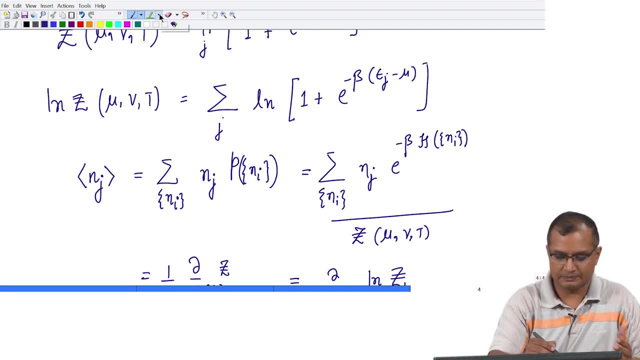 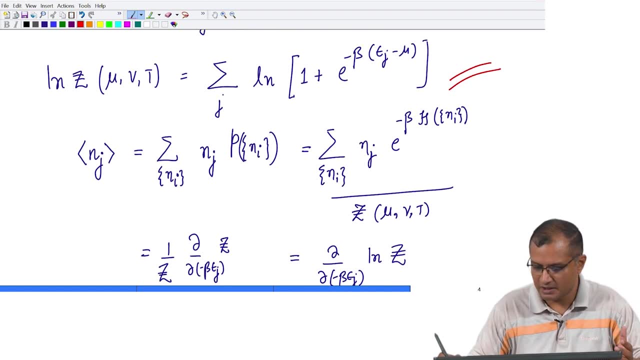 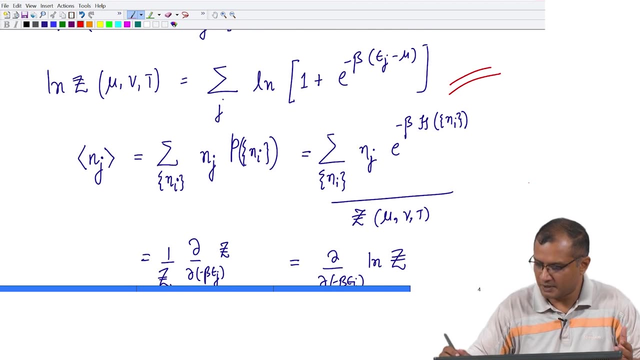 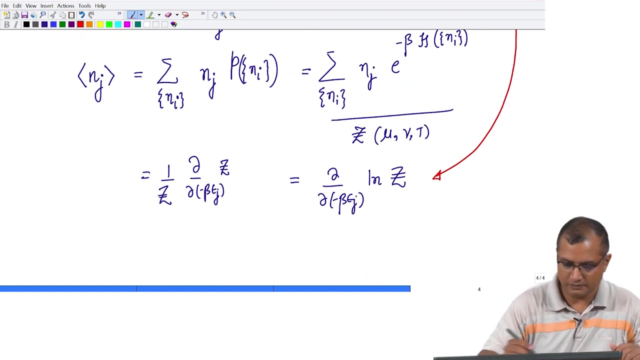 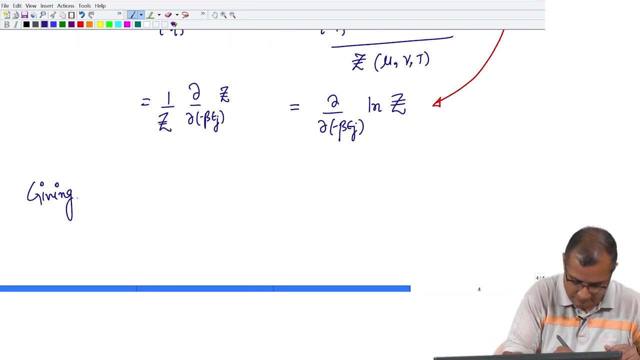 the system of fermion. So I am going to use this expression for ln z. ok, So plugging this expression in ln z, what do I get? So I am going to plug this for this ln z. ok, So it will give me what is my left hand. 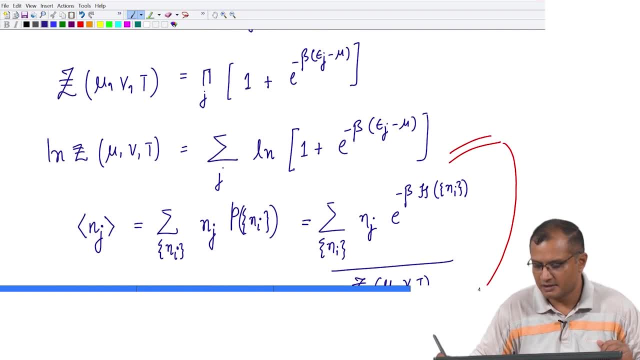 side, and please look at ln z here. So in this summation only the j over a. So let J th term will contribute. J is running from 0 to infinity, the infinite energy levels in our system of that. out of those infinite levels, only one level, J, will contribute to this derivative. 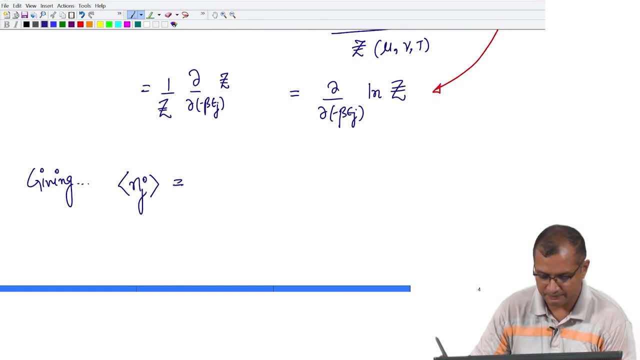 and that will give me 1 plus e raise to minus beta in the denominator and I will have a e raise to minus beta E j minus mu in the numerator. and just multiplying and dividing by a common factor, I can write this as a e raise to beta E j minus mu in the numerator. 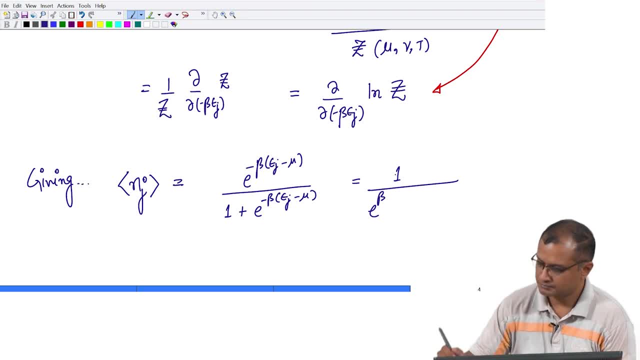 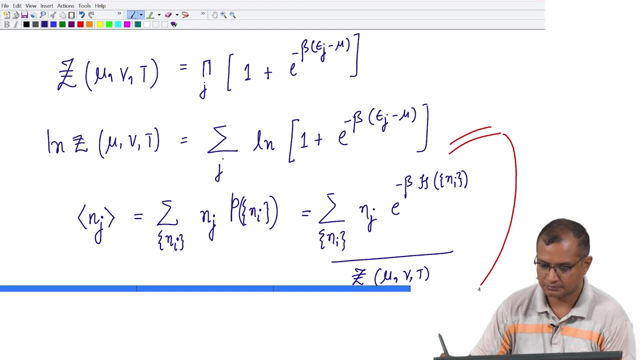 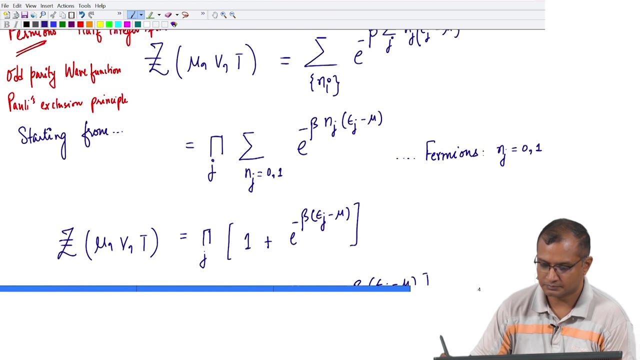 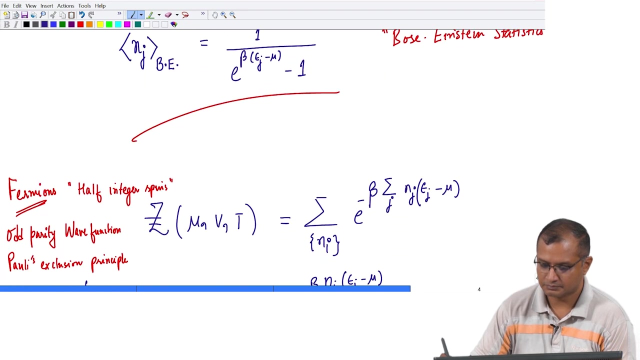 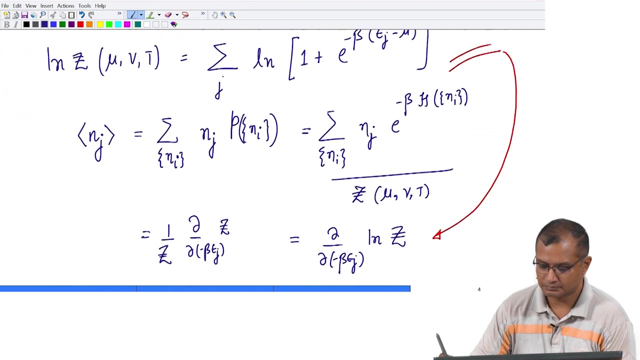 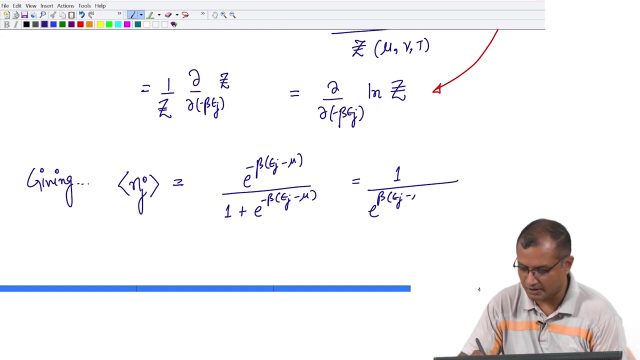 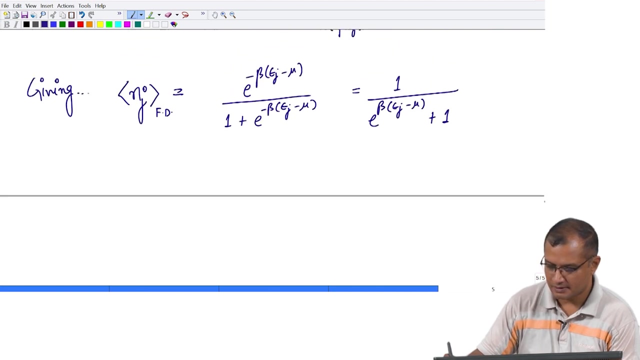 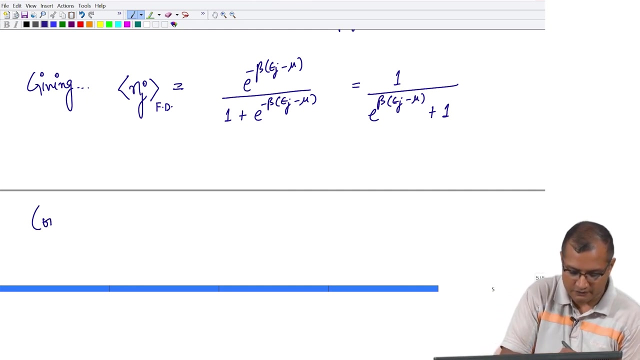 All right, E j minus mu plus 1, ok, So then, just to remind ourselves, this is nothing but Fermi Dirac statistics, So I can write this as combining both the results of the Fermi Dirac and the Bose Einstein statistics. I can write down combining both of them. 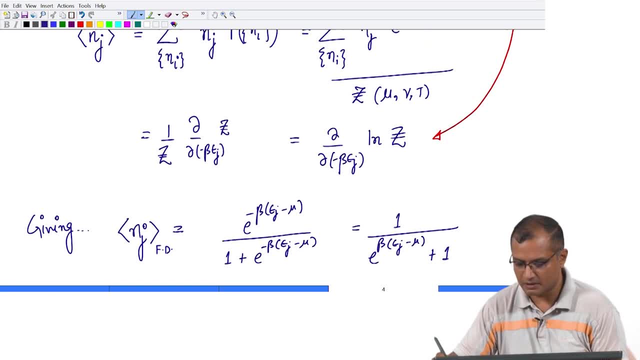 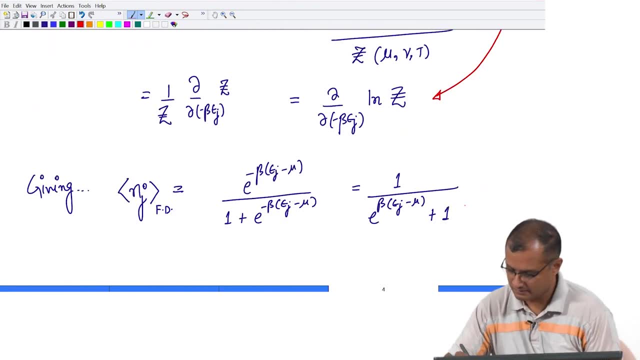 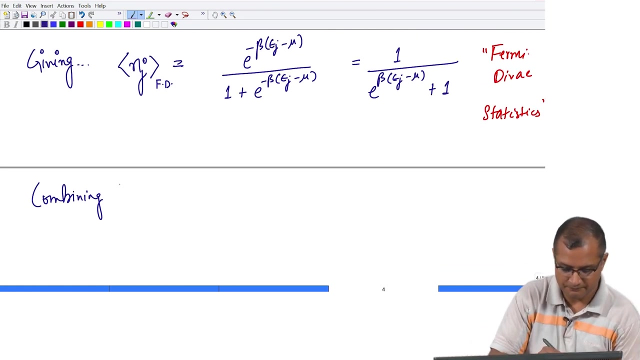 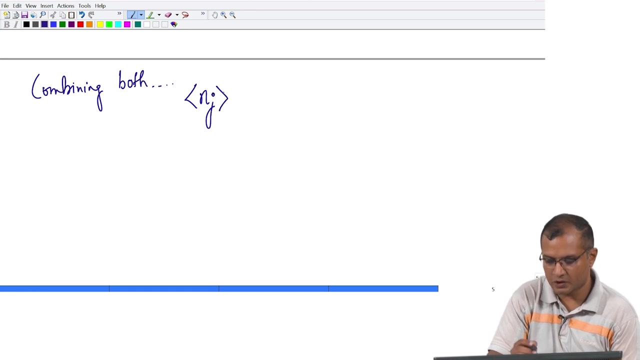 So let me call this as some equation. So far, yeah, combining. So I am going to call this as Fermi Dirac. So, combining both of them, I can finally write down a single expression for the average occupancy of the J th energy level as Fermi Dirac or Bose Einstein. as I can, in fact it is better. 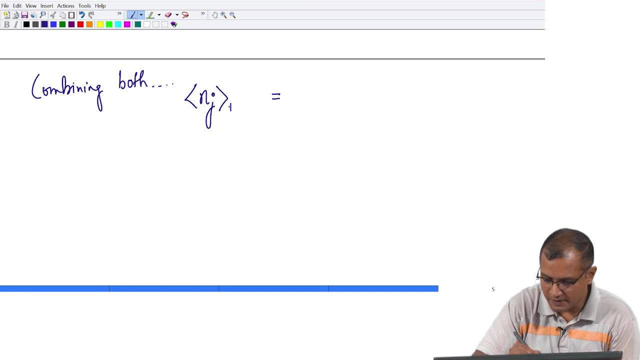